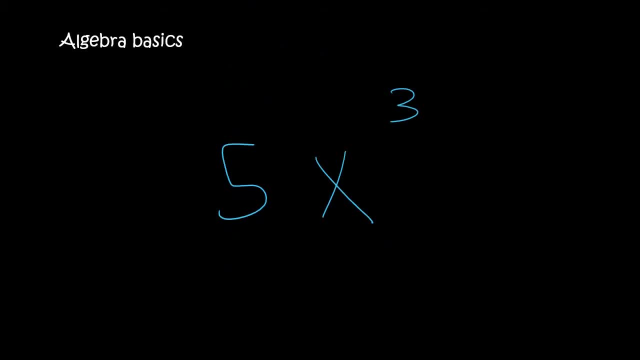 variable and exponent: Coefficient. variable and exponent. Coefficient. variable and exponent. Variable exponent. So just to make sure you've got that, maybe you pause this video. The x is the variable, the 3 is the exponent and the 5 is the coefficient. Now in algebra you could have sums. 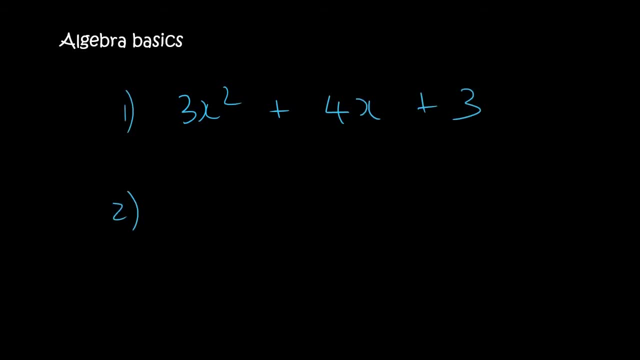 that look like this: That's number 1.. You could have something like that, or you could maybe even just have that. So this one at the top has 1,, 2, 3 terms, so we will call this a trinomial, This one. 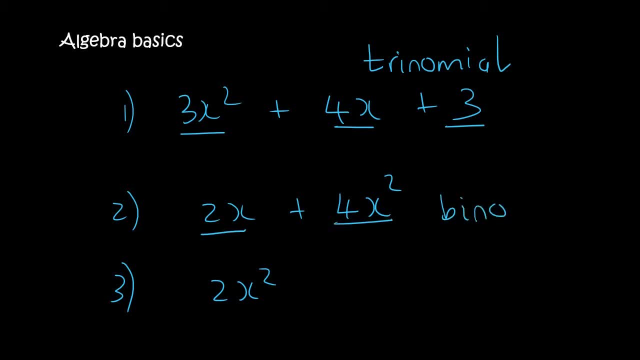 has 1, 2 terms, so we'll call that a binomial. You know, like a bicycle, it has 2 wheels, This one's like a tricycle, it's got 3 wheels, And when you only have 1, then we call it a monomial. So all. 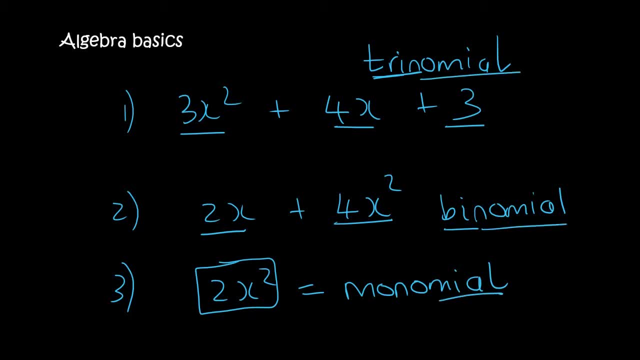 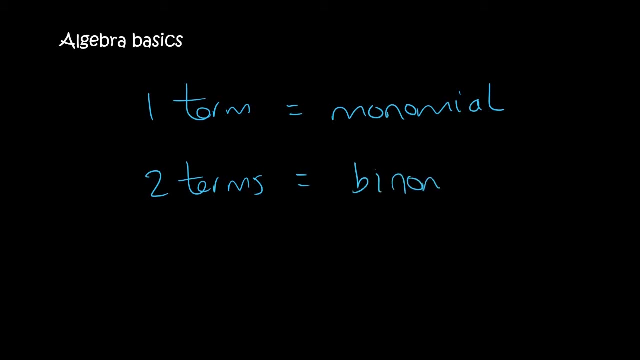 of them end with 1.. Then you just got tri-bi-mono. So if it's 1 term, that's monomial, 2 terms binomial And 3 terms will be a tricycle, so it's a trinomial. So this is your bicycle trinomial. and then you've just 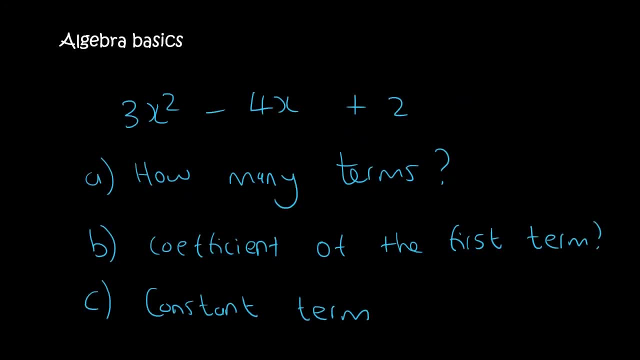 got to remember mono, Alright, so maybe if you want to pause this video and then you can try this one. So here we're saying how many terms? Well, that's 1, 2, 3.. So that'll be 3 terms. Then they're saying the coefficient of the first term. So we look at 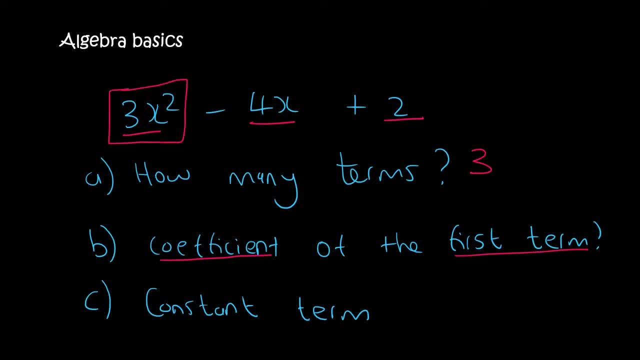 the first term, and remember, the coefficient is the number in the front, And so that will be a 3. Let me just write that there in case it doesn't fit in. And then constant term. Okay, so we said that if you have something like 3x squared, the 3 is the coefficient. 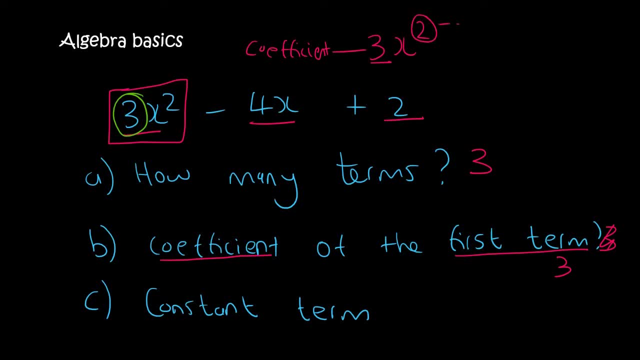 The 2 is the exponent And the x is the variable. Now the word vary means change. If something can change, okay. So in number c they're asking you for the constant term, So it's the one that can't change. So it can't be this, because that has an x and that x can change because it's called a. 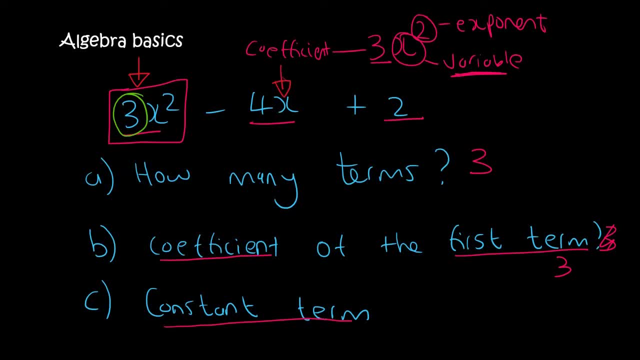 variable. This one has an x, so it can't change because it has a variable. And then you've got, but this one does not have an x, And so this is called the constant term, because it will always be 2.. Whereas the one in the middle, for example, if x is 1, then that becomes. 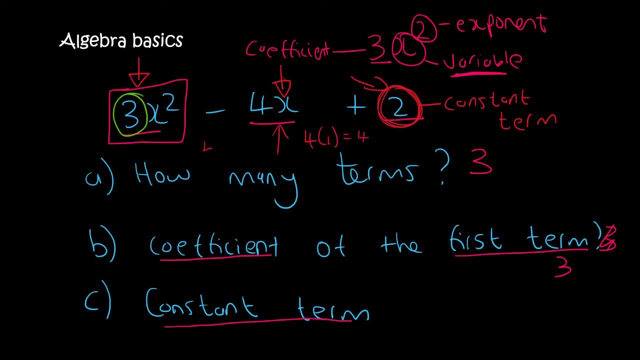 4 times 1,, which is 4.. And if x was 2,, then it would become 4 times 2,, which is 8.. And so this whole term can change. However, this 2 will always be a 2. So it's called the constant term. 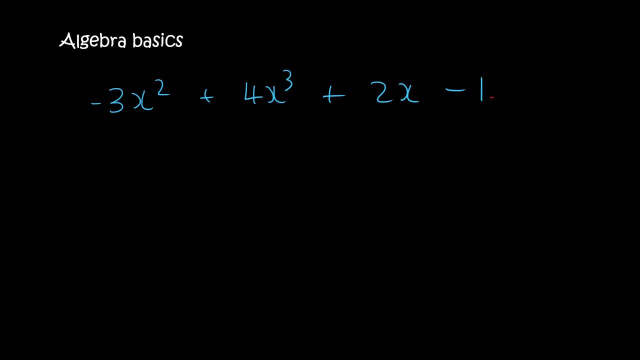 Here we have something that has four terms, So if it goes more than three, if it has more than three terms, then just call it a polynomial. Poly means many, So if it was one term, remember that's a monomial, 2 is a binomial And 3 is a trinomial. If we go further than that, 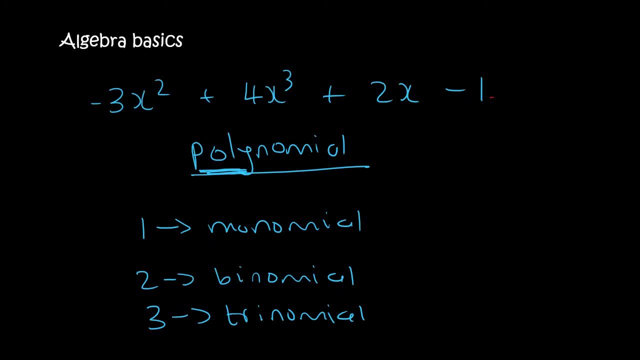 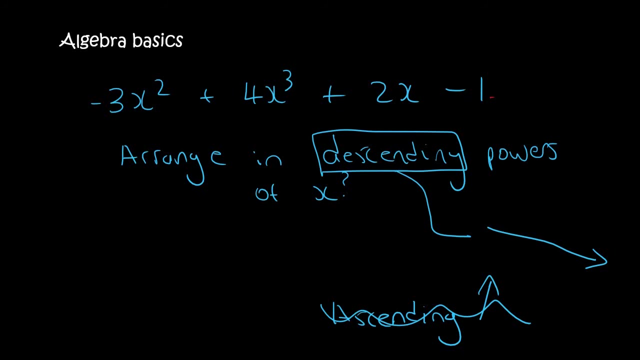 then we just call it a polynomial, because poly means many. Here's a question: Arrange in descending powers of x. So descending, you need to know that that means going downwards. If we said ascending, then it means going upwards. So they say: arrange it in descending powers of x. Powers are these things? They're also called: 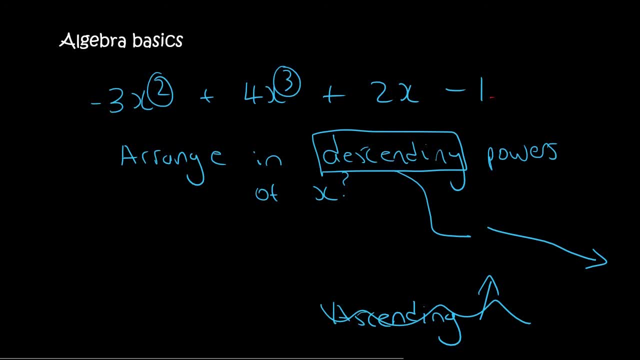 exponents. So descending means from biggest to smallest. So this one has a 2.. This one has a 3.. This one seems to have nothing, But remember, that actually means it has a 1.. And this one really has nothing, So that one's got a 0.. So the largest one would be. 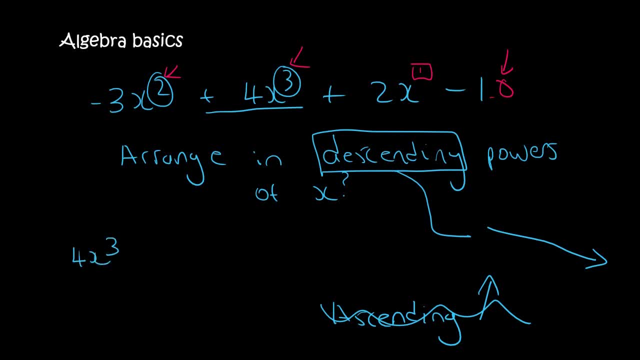 this one, So you put that one in the front. The next one is the 2. So you write all of that like that. The next one is this, And then, lastly, at the end, you've got minus 1.. Let's practice this. 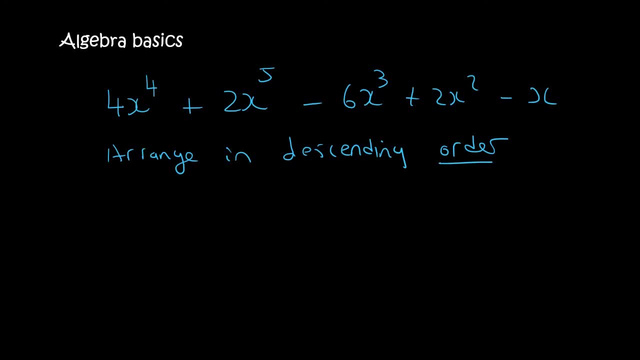 a bit. So here we're going to arrange this in descending order, And they're always talking about exponents, They're not looking at the numbers in the front And then remember if there's nothing there, then it's a 1. So descending means from biggest to smallest. So that's the